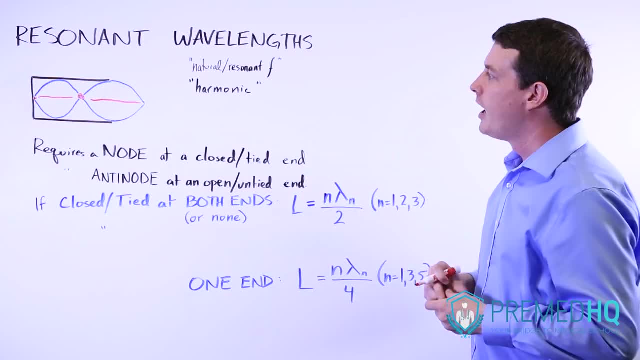 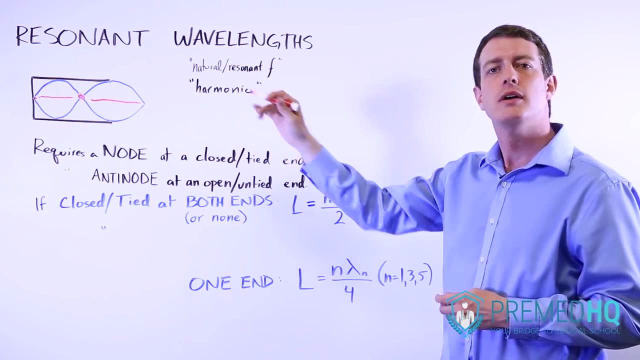 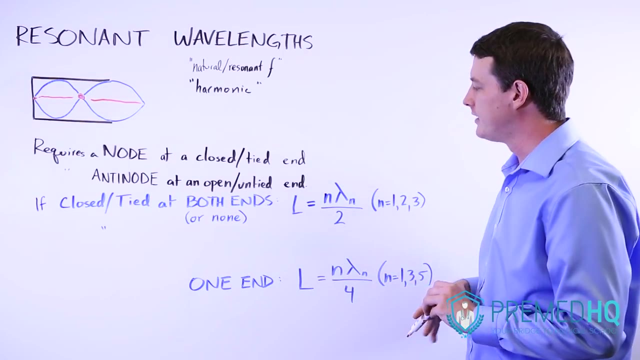 order for harmonic or resonant wavelengths to be exhibited, and you need an anti-node, which is where the waveforms are as far apart as possible whenever it is at the open part of the pipe or the untied end of that string. If you know the nature of your system, then you can calculate the wavelength. 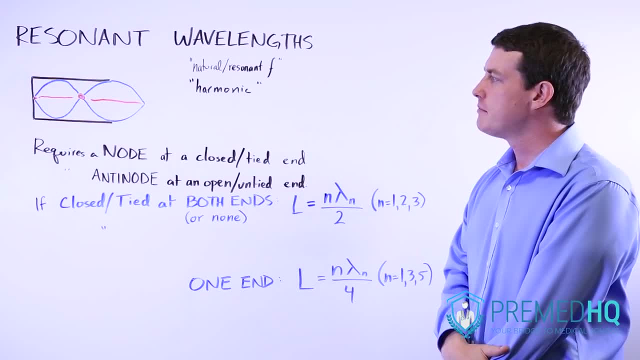 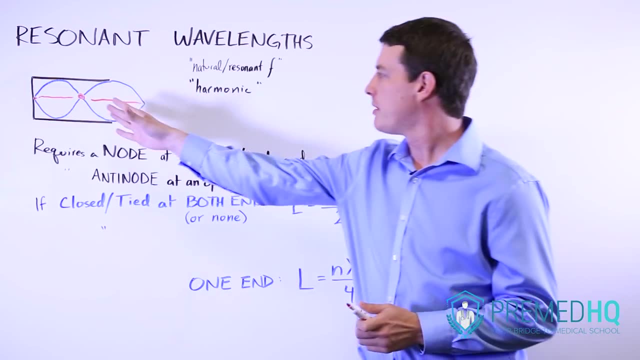 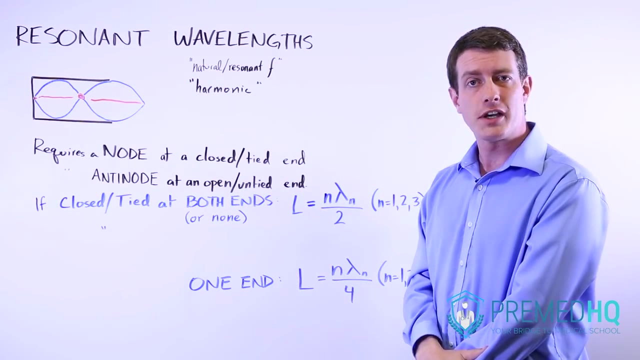 of these harmonic or resonant wavelengths simply by knowing the length of the chamber, and usually this is done in the case of pipes, where you know how long the pipe is and you know whether it's open or closed at each end. You can also do this with a string that is tied at both ends, such as with a. 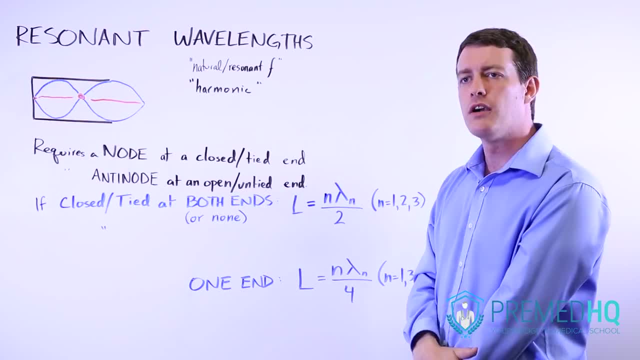 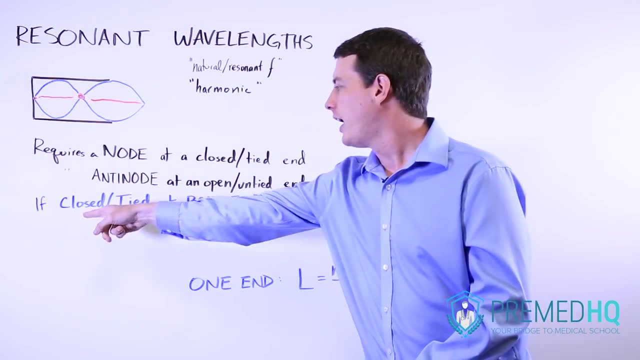 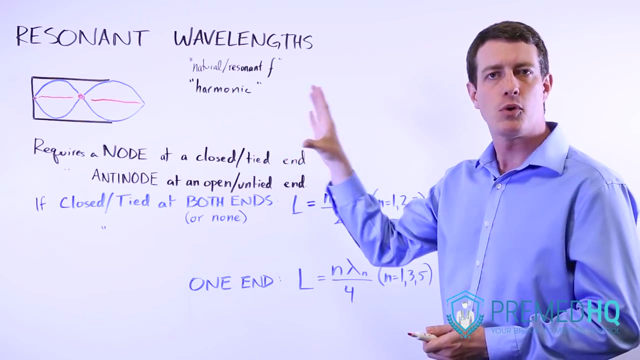 guitar or any string instrument. These are all cases where harmonic resonant wavelengths will appear and the calculations that you use. if it is closed or tied at both ends or neither end, then you use the formula that the length of the pipe or the length of the overall waveform, for example the length 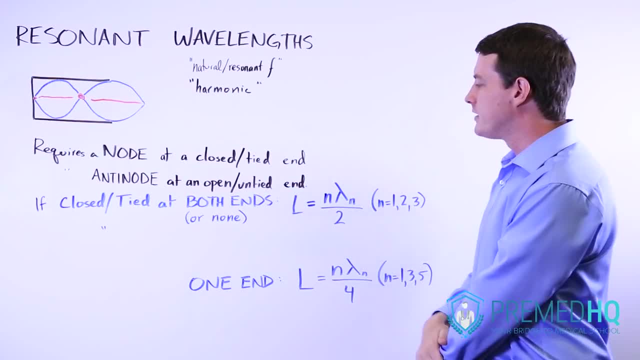 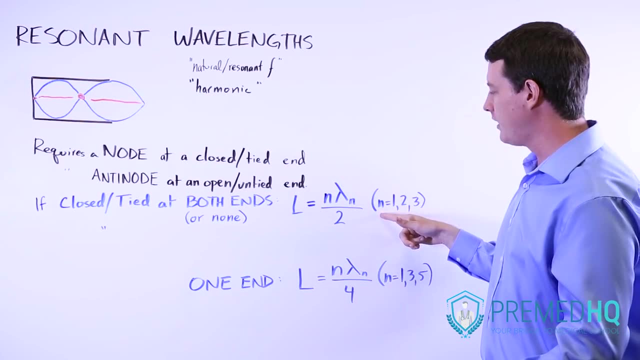 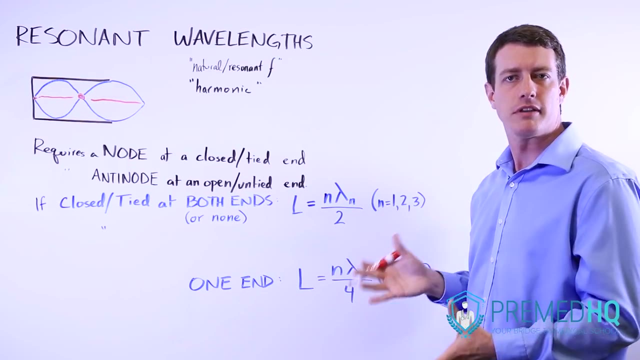 of the distance between the two ends of the guitar string is equal to n times lambda sub n divided by two, and for this you use n with any value, any integer, one, two or three, and that will give you all of the various harmonic wavelengths that you encounter with that. So if it's closed and tied at both ends or at neither end, then 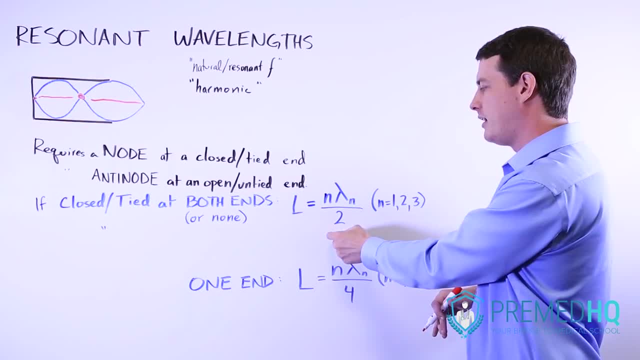 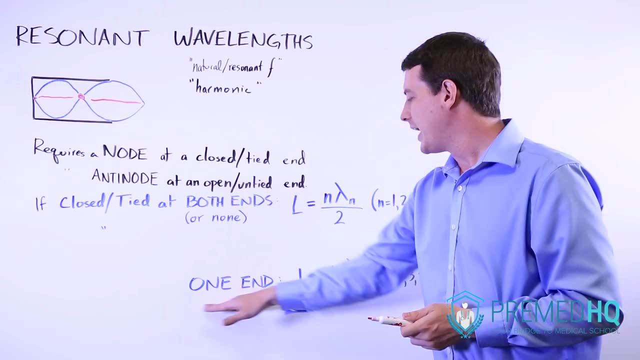 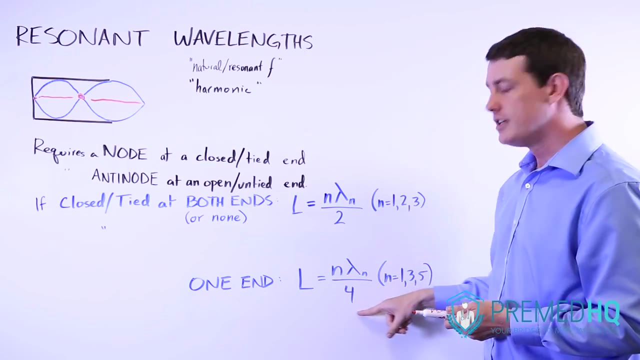 you use this formula: l equals n times lambda sub n times divided by two, and the lambda here represents the wavelength. Now, if it's closed or tied at one end, then you use a different formula. the length of the pipe or chamber equals n times lambda sub n divided by four. 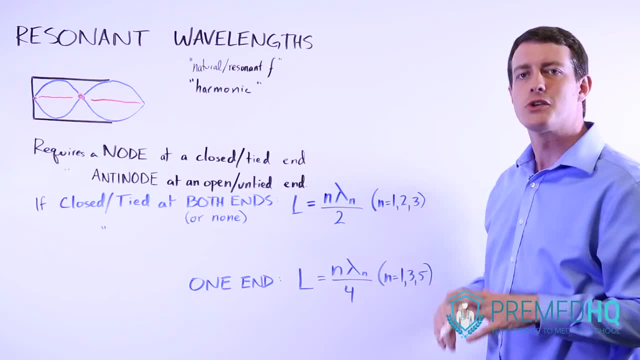 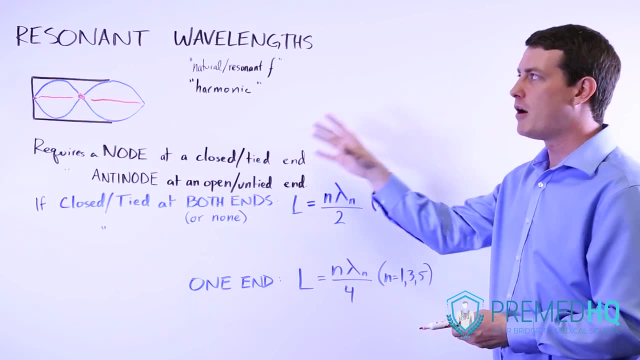 but in this one you skip every even numbered integer, so it's only odd numbered integers- It's one, three, five and seven that can be used to calculate your harmonic or resonant wavelengths. in this example, where it is tied or closed at only one end, 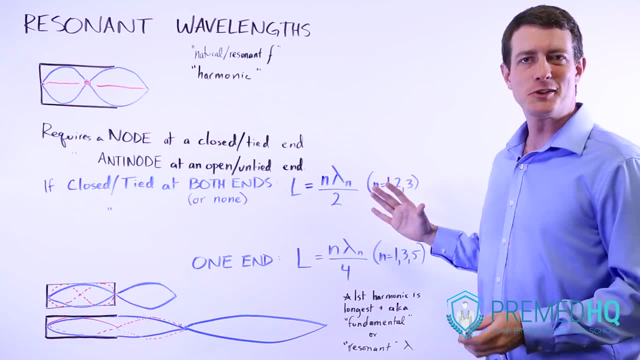 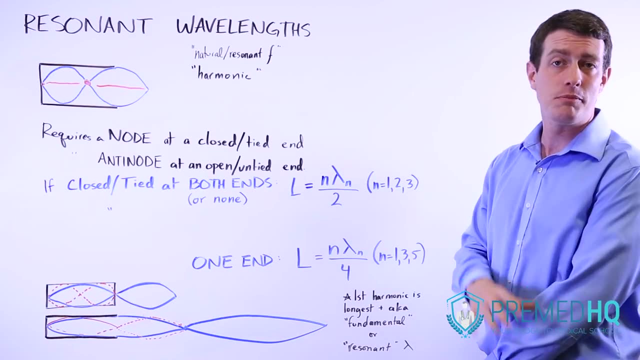 At first glance, these formulas may seem somewhat random and counterintuitive, but I've drawn two illustrations here to show you that there actually is a reasoning behind them, and this can also help you remember them if you're forgetting which denominator you should use for each one. and 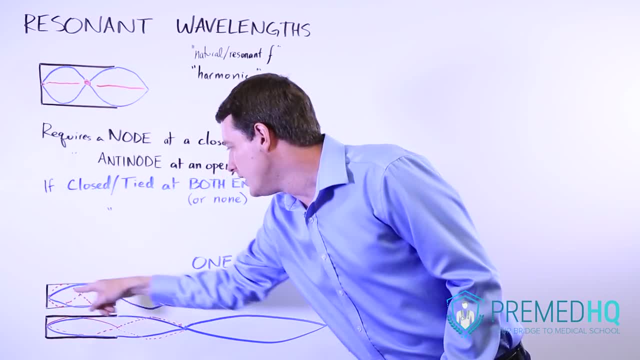 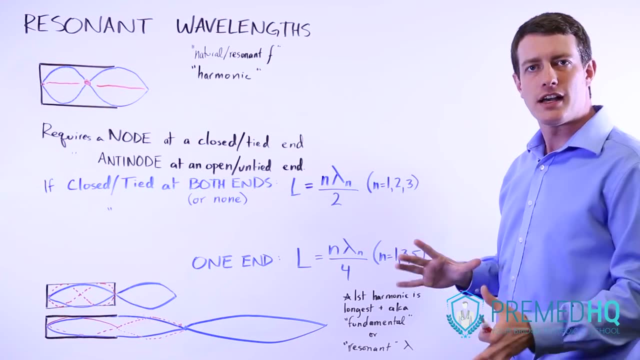 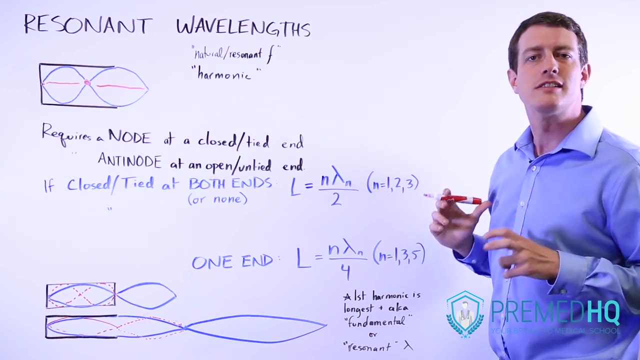 so let's remember that if it has a closed end at both sides, then what you need is a node at both sides, and so the longest wavelength that satisfies those requirements, the longest harmonic, which is also known as the first harmonic, the fundamental or the resonant wavelength, that will be something. 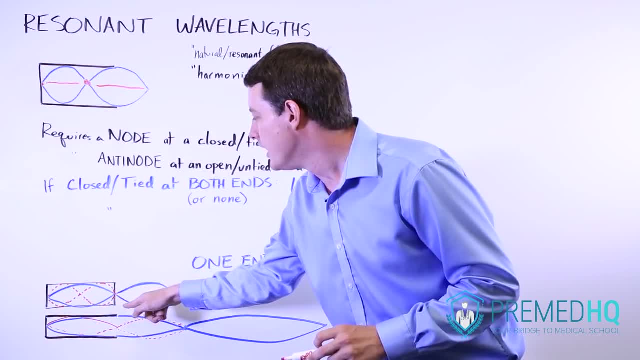 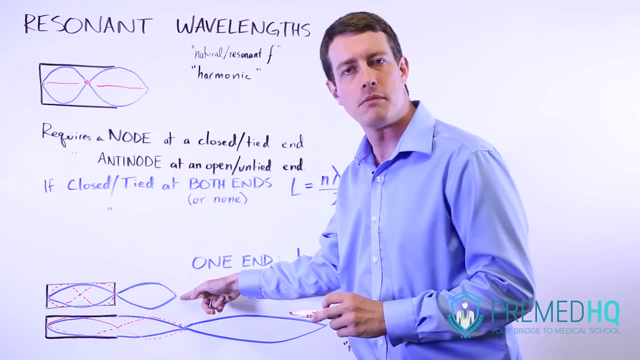 that is required to have a node here and the longest thing that does that is going to be twice as long as the chamber. so if you draw out this whole waveform, from when it rises to when it falls, to when it comes back to that position, notice that it is twice as long as the chamber. 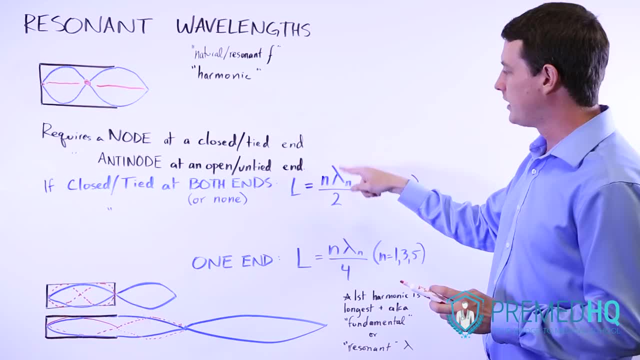 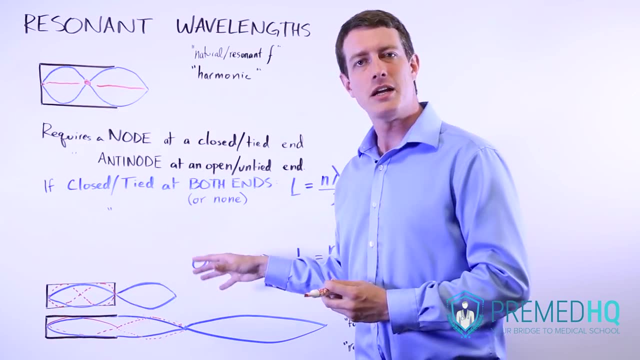 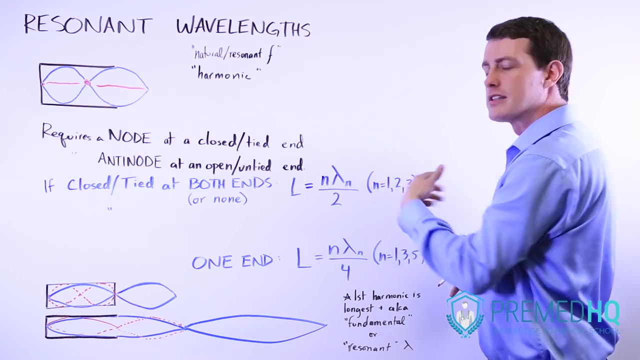 so the fundamental one, which is going to be n times Lambda sub n divided by two, it's going to make sense that the fundamental one is twice as long as the chamber, and so if you were to use n is equal to one, because it's the first harmonic Lambda sub n is going to be the length of the. 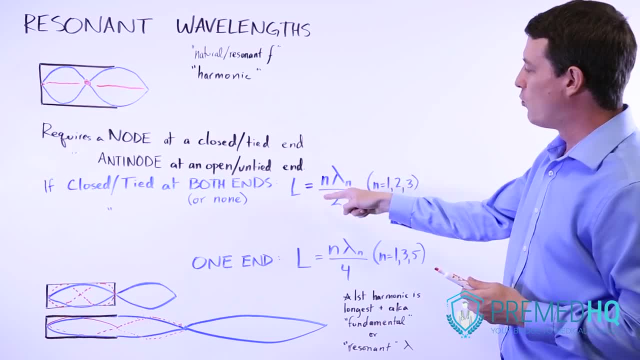 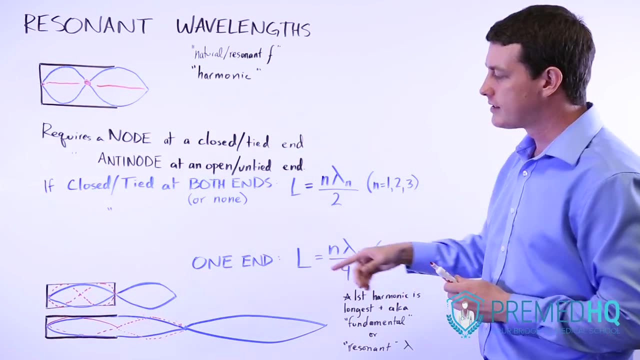 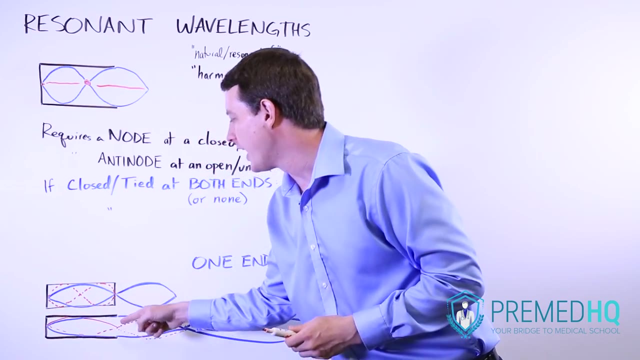 first harmonic, the wavelength of that harmonic. so if you multiply one by that wavelength and then divide it by two, that will give you the length of the chamber. now notice that down here in this example, where it is open at this end, the first one that satisfies the requirement of having a node here and an anti-node at the open end is going to be a wave. 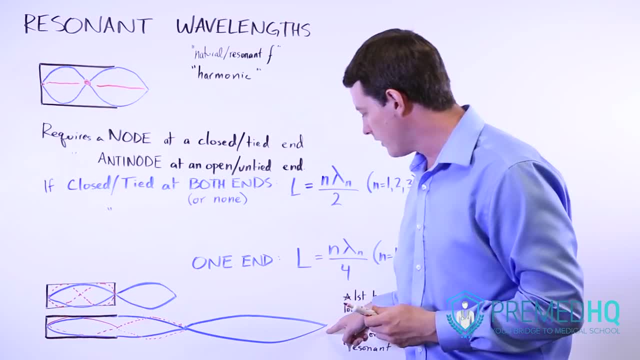 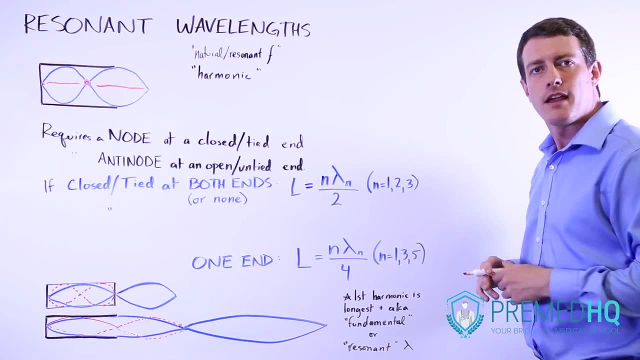 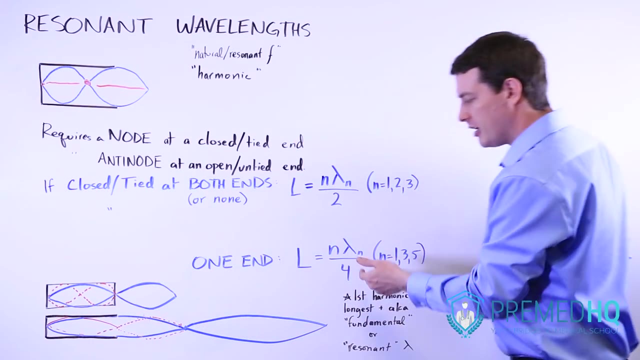 that rises to here, comes back to the middle, goes down here and then reaches this position again, that one is going to be four times as long as the chamber, and so if you were to use this same formula, using n as one Lambda, sub n as the wavelength of this, you would have to divide that by four in order to. 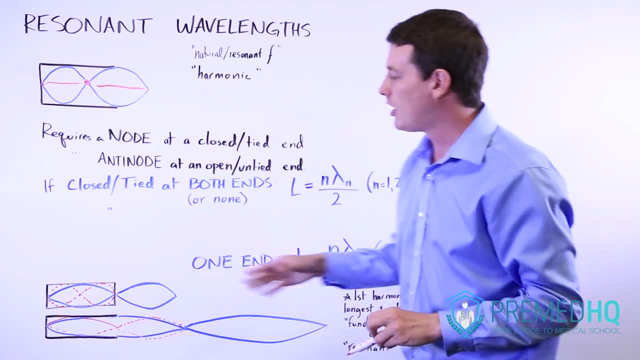 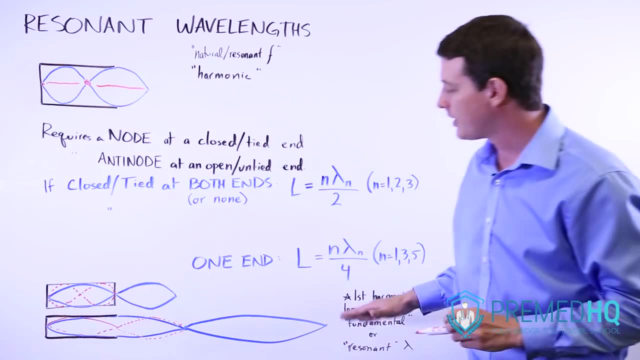 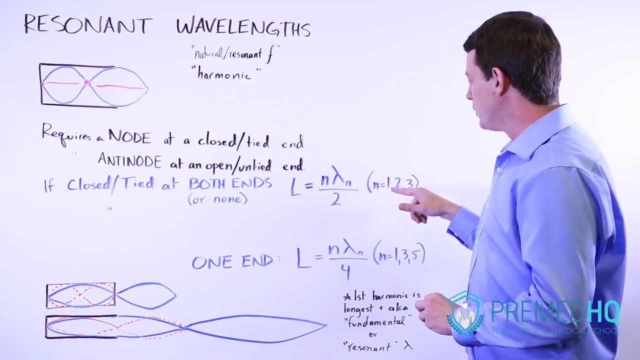 get the length of the chamber. so it kind of makes sense that if the longest thing that satisfies this requirement of having a node here and an anti-node here, if that thing is four times as long as the chamber, you would have to divide by four. now the other question: why do you use every? 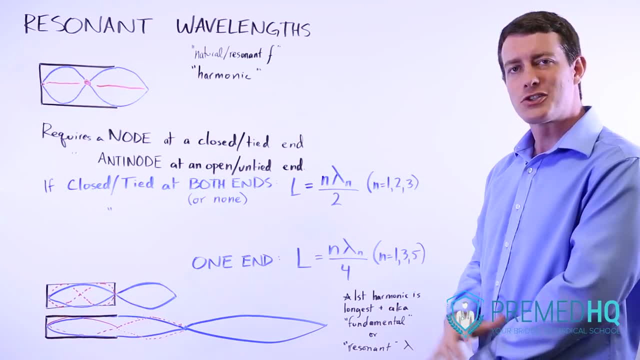 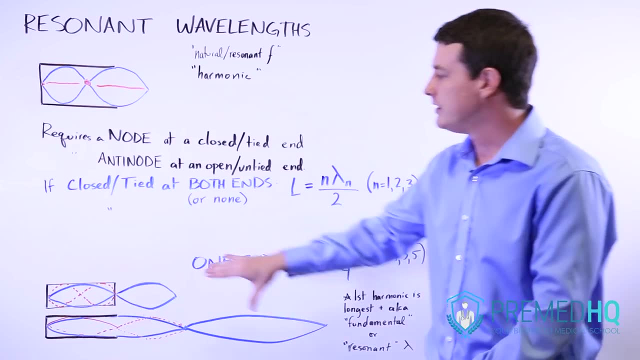 integer here and every other integer here. that one is fairly straightforward too. notice that in red I've drawn something that is half the fundamental wavelength here and that in this example, where it is closed at both ends, you end up getting a node at this end here, which is: 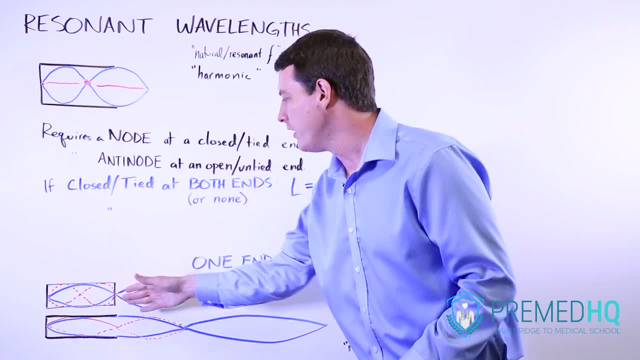 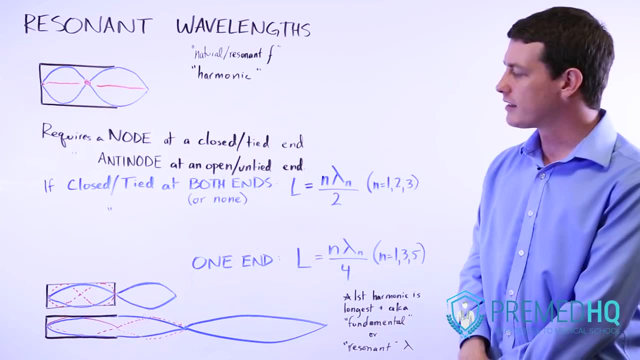 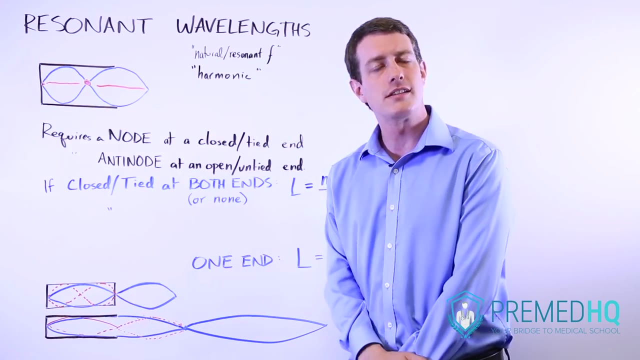 what you want. that is something that is half the wavelength of this first fundamental wavelength. now here, if you're drawing something that is half of the fundamental wavelength, notice that it produces a node at this open end and that does not satisfy the requirements for resonance, and so that can help you remember that every sort of permutation of this longer one, 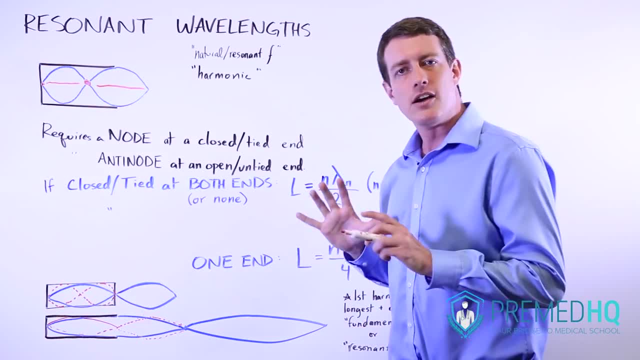 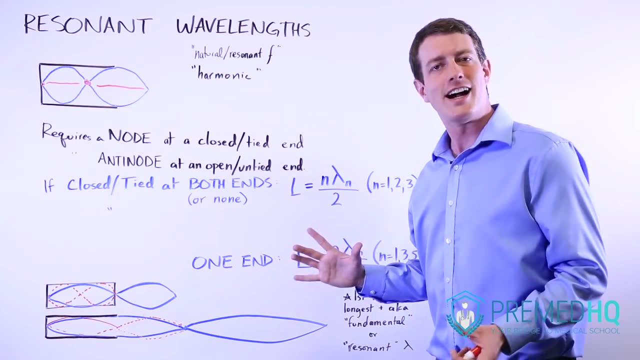 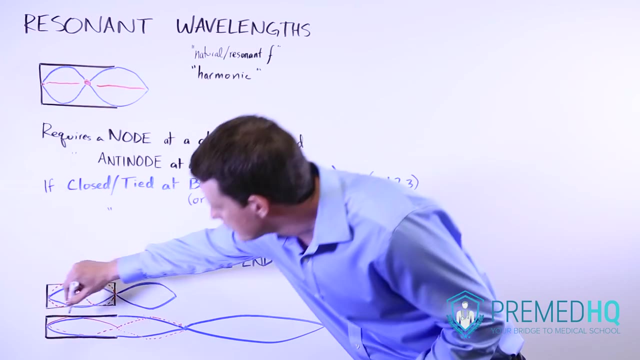 not every one of those is going to satisfy the harmonic or resonance equation that you need, and so that's why, with something that is open at one end or is untied at one end, you end up skipping every even numbered integer. so the next one that will satisfy the requirements for resonance here. 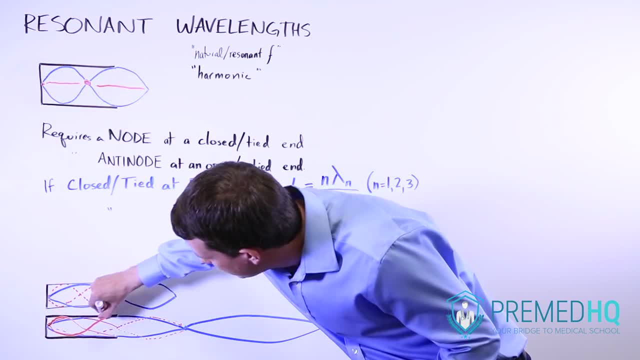 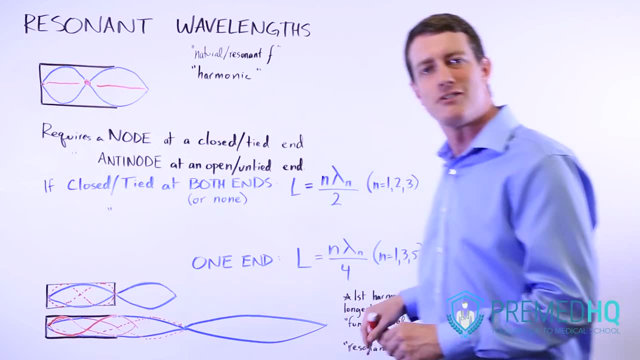 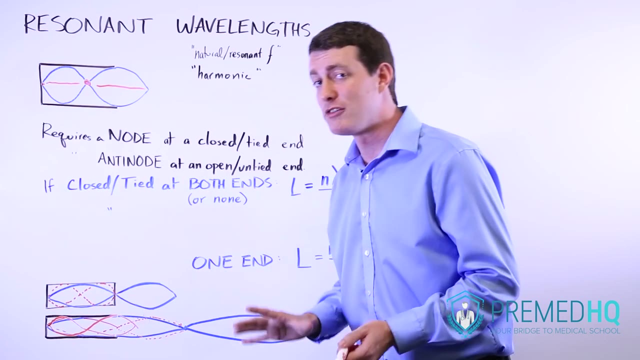 will be something that goes up and down there and then goes down and up here. that is is what satisfies an anti-node, but notice that this isn't even close to being half as long as the fundamental. so just remember that if half of your fundamental one doesn't satisfy that requirement, 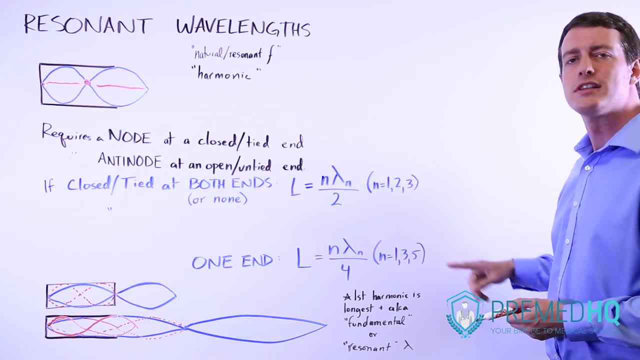 for having an anti-node here, then you can't just assume that every single integer will yield a harmonic. 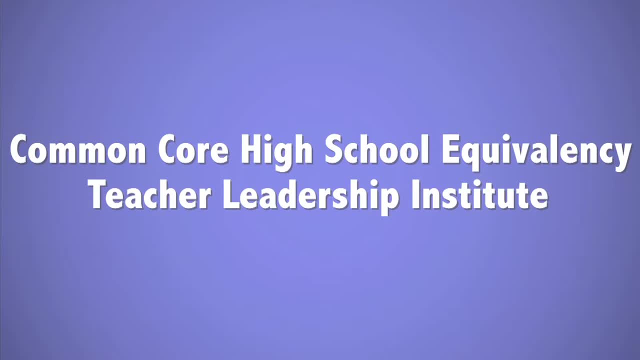 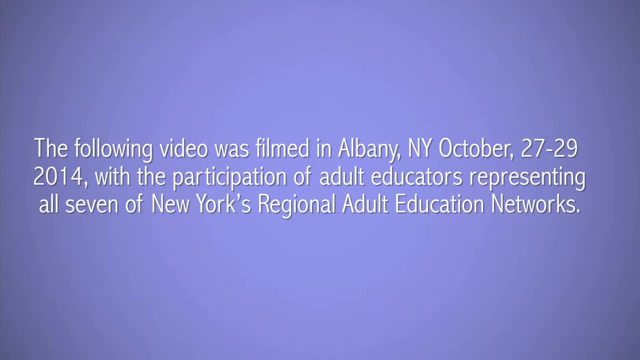 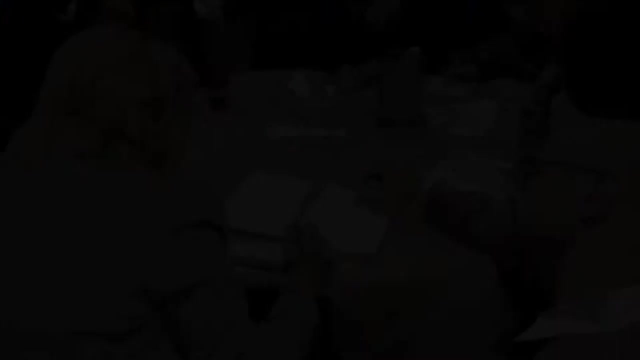 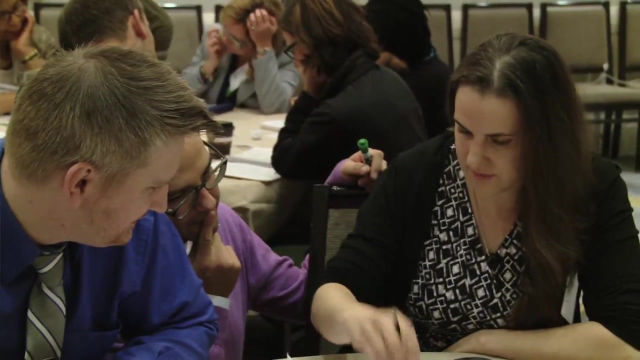 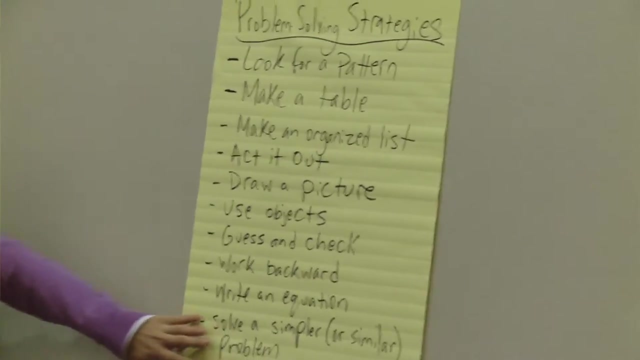 Once we give students these problems that require more than just having something memorized. they need tools. Often with students, I use a list written by a great educator named Marilyn Burns: The problem solving strategies. on that to give you a sense: drawing a picture making. 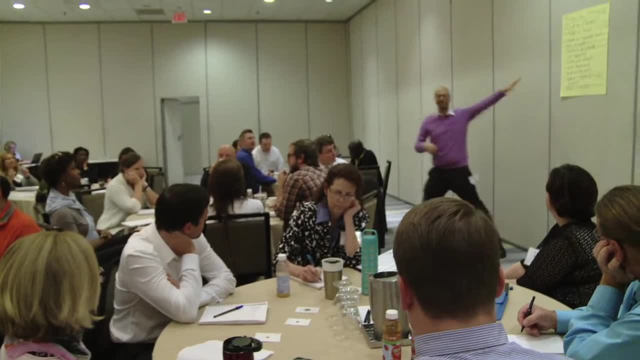 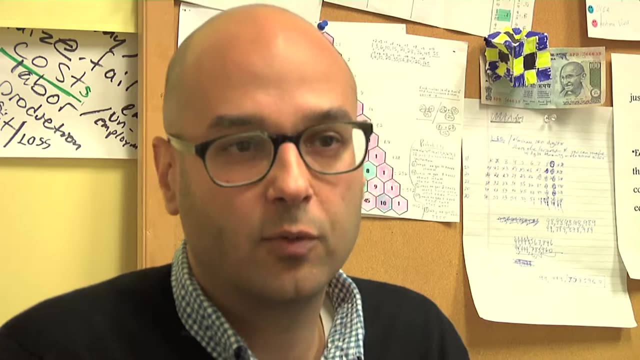 a chart or a table making an organized list, looking for a pattern. They need to learn to persevere. You try something and it's hard and you struggle through it. One way that we can keep that struggle productive is to help students build a toolbox of problem solving. 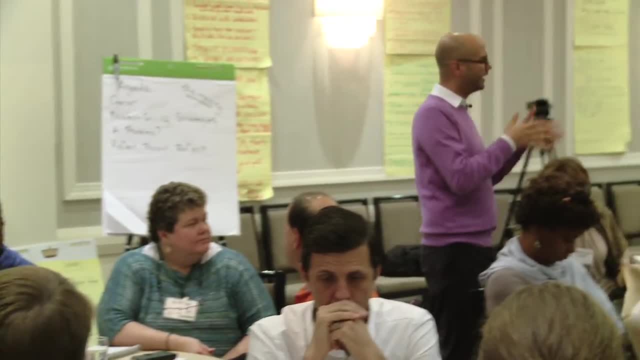 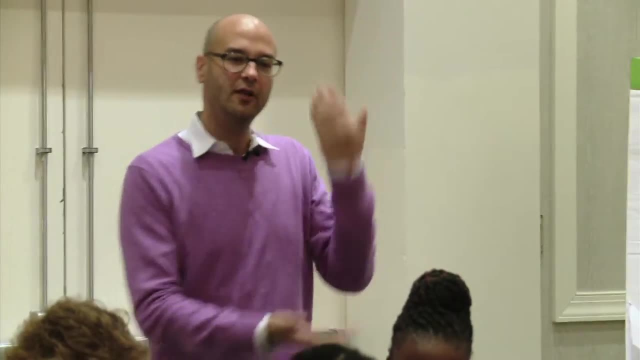 strategies. Today in the morning session we're going to do a problem that fits that, but again we're going to be focusing on the problem solving and how to create a problem solving atmosphere in your classroom. So there's a problem called the bicycle shop. The bicycle shop problem is essentially someone.